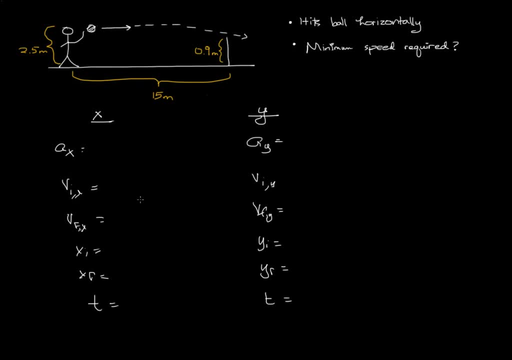 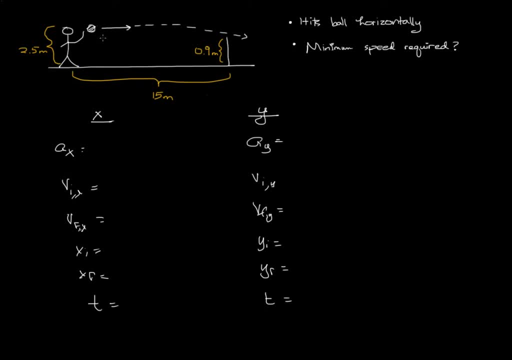 know. So what is the acceleration of this ball in the x-direction? And again, unless there's some fuel coming out of this ball which is going to cause this ball to accelerate in the x-direction, we pretty much can assume that it's zero meters per second squared. 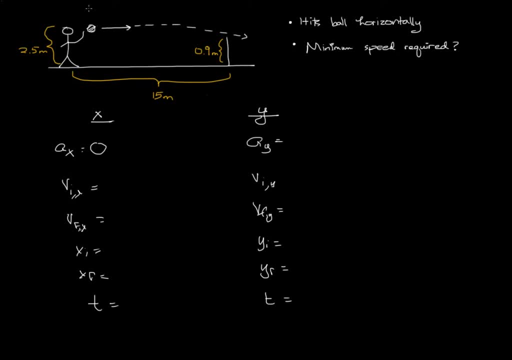 On the other hand, gravity is this mysterious force in the universe that is always causing objects to accelerate downwards at a rate of 9.8 meters per second squared, and since it's down, it is negative. So gravity is acting on this ball and that ball will. therefore, 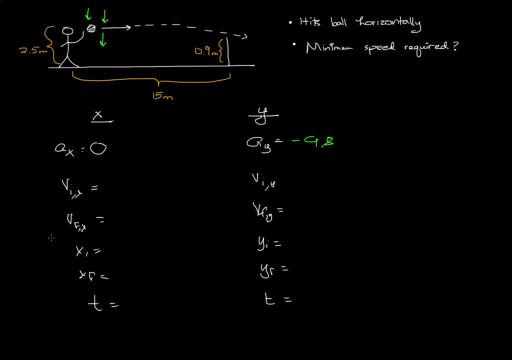 accelerate downwards at a rate of negative 9.8 meters per second. squared Alright. Now what is the initial velocity in the x-direction? And that's what we're trying to figure out right: The minimum speed required to cross this net. 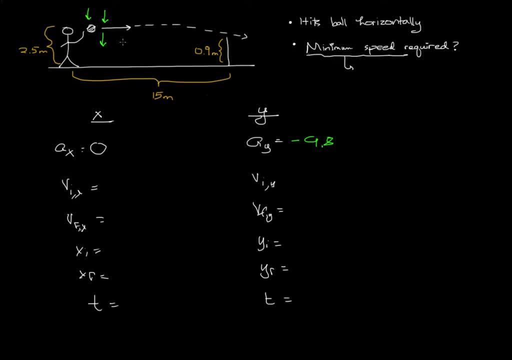 So this is asking: what is that minimum speed you have to give it initially? So we're trying to figure out that V initial. So we actually don't know this. That's our goal: to figure this out. So what about V initial in the Y direction? 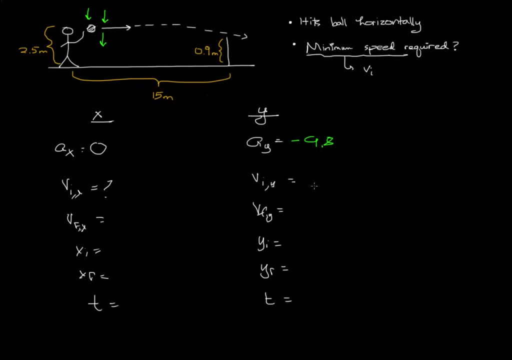 And you might initially be tempted to think that we also don't know V initial in the Y, But actually the problem tells you that we are hitting the ball horizontally right. We're giving a complete horizontal initial velocity, So we're not trying to hit it as a 2D vector which would have an X and Y component. 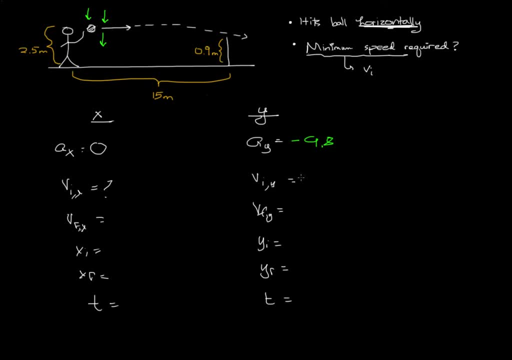 Or we're not trying to hit it completely up, completely horizontal. So therefore the initial velocity in the Y direction would actually be zero. So it's very important to read physics problems carefully, because every word actually kind of matters, right If you kind of casually ignore this word horizontally. 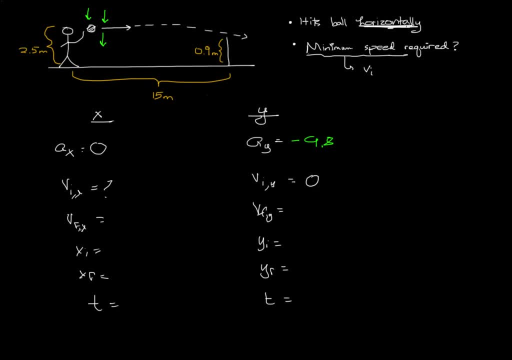 this could cause confusion And that would mess up the problem. So make sure you just read it carefully and look for these clue words, right, That we've shown in previous videos as well, and this is another one. So just look for these kind of cue words like this: 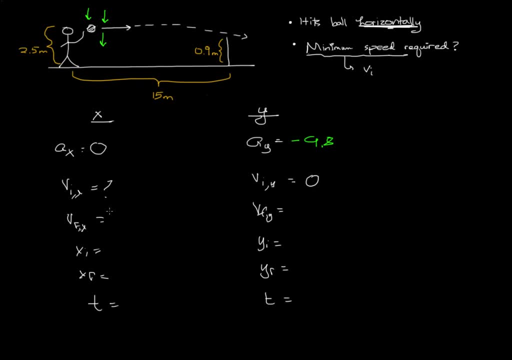 Alright, what is the V final? in the X direction. So we don't know what it is necessarily, but we know that, since there's zero acceleration and we are starting at some velocity which is unknown, we know that the final velocity 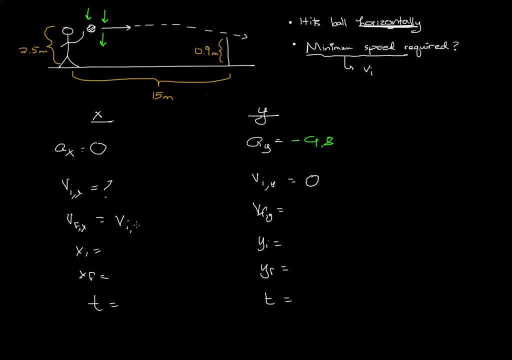 the initial velocity in the X is still going to be the same initial velocity in the X direction, right? So for those of you who haven't seen the previous videos, I'll just quickly recap that if you're starting off at some initial velocity and you have zero change, right. 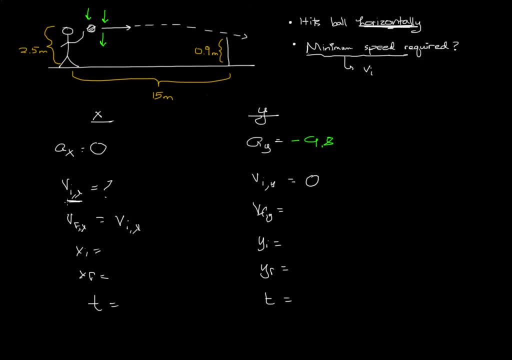 Because acceleration is just a change in velocity. So if you're starting off with something and you don't change it at all, you end up with that exact same thing. So even though we don't know what we started off with, we know that we're going to end up with that initial velocity in the X. 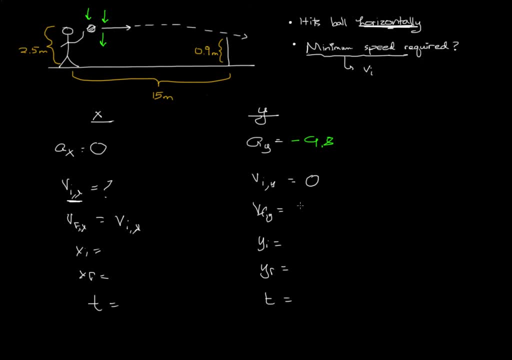 So that's kind of neat On the Y side. we just don't know what that final velocity is in the Y direction because we're starting off at zero. We are changing negative 9.8 meters per second, every second. so therefore we have no idea what it is when it reaches that point. 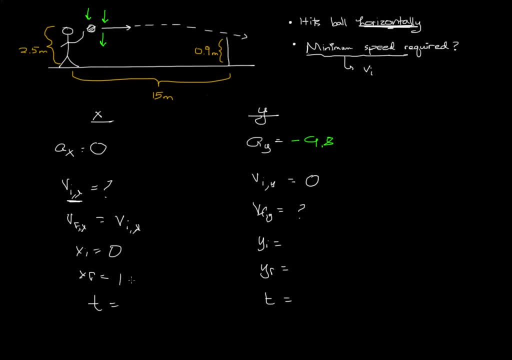 Alright, the X initial is zero, the X final is 15, and the time is unknown. The Y initial is 2.5, because we're starting 2.5 meters above the ground. we end 0.9 meters above the ground. So that's what we're looking at and what is the time again is: 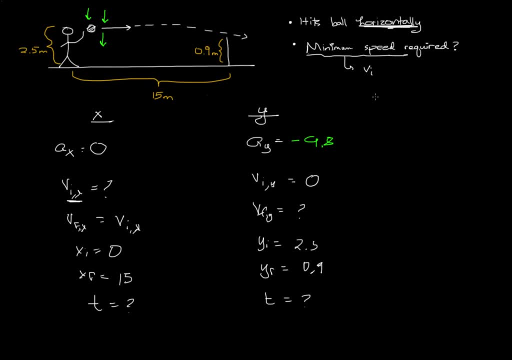 unknown, Great. so our goal is really to figure out not just v initial, but really v initial comma x, because there is no v initial comma y, it's zero. So, generally speaking, thus far, whenever we've needed a variable like v initial comma x, we typically go directly to the x side right, because 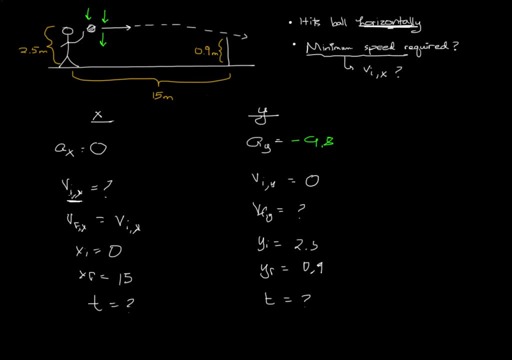 if you need v initial and x. I pretty much stressed: always stick to x or y separately, don't mix them together. So that's the natural instinct. so let's see if we can do that. so we need v initial in the x direction. so what kinematics equation can we use to get v initial and the x? and the problem is: 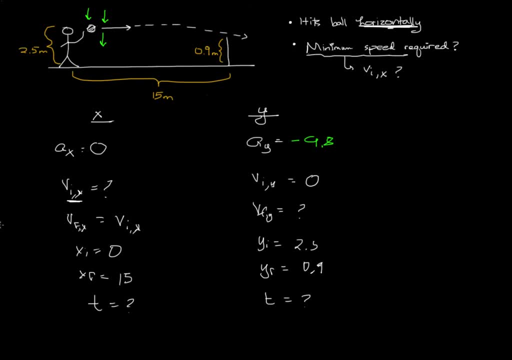 that we don't really have a lot of information on this x side, right? so let's see, can we use v final? oh, whoops, let's see, let me draw it here. so can we use v final? x equals v, initial x plus a, x, t. can we do that? we can't right, because we don't really know what v final in the x. 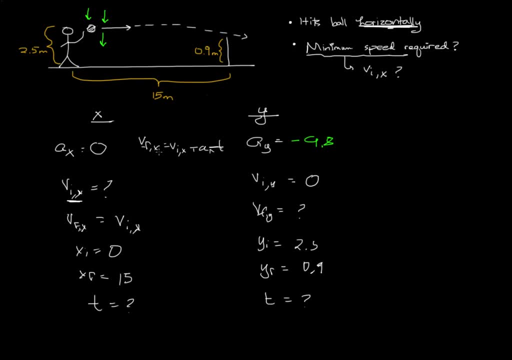 direction is. we know it's the same as v initial in the x, but then that'll just kind of cancel everything out and then you'll have 0 equals zero, so that doesn't work. Can we use our next kinematics equation, which is delta x? 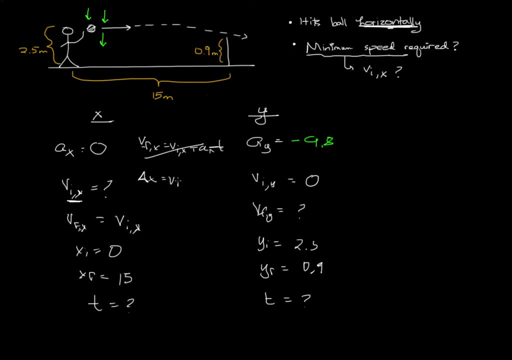 equals v i x t plus one half. oh, that's getting messy: v i x t plus one half a x t squared, And the problem with this one is that we don't know time right, So we're kind of stuck with this as well. so that doesn't work, And our last option is v. 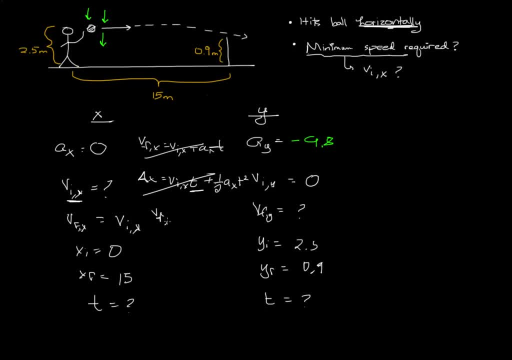 final in the x direction squared minus v initial comma. x squared equals two a delta x. And again we can't do this because we really don't know. well, we know v final in the x is the same as v initial in the x. so if we plug that in we're just going to get zero equals zero. So again, 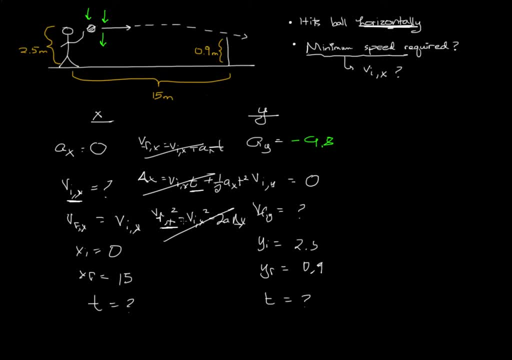 all three of these do not work. So this is our last option and we're kind of stuck with this as well. so that doesn't work. So this is why I wanted to do this problem, to highlight one more way they can kind of 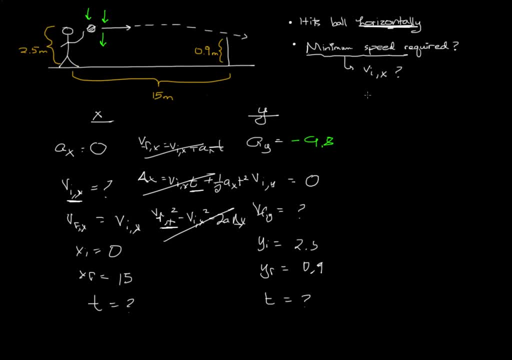 trick you on exams and stuff is they can give you a problem like this where you need something, let's say, in the x direction, and nothing works out. So a lot of people get puzzled at this point and kind of give up. But you have all this information on the y. 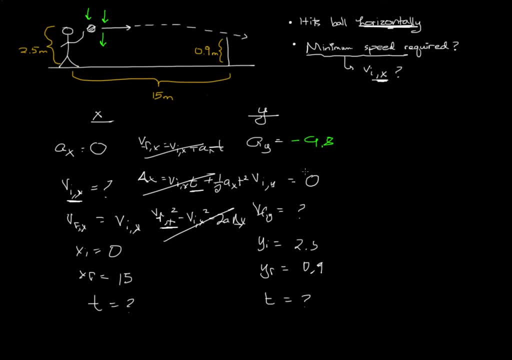 side right. But I just said you can never mix the two, which is true. so you can never say: when I say don't mix them, I mean you can't say v initial v, final x equals v, initial x plus a yt. You can never mix x and y in the same equation. That's a big no-no. But 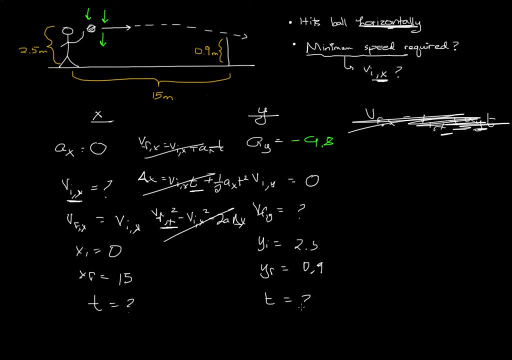 what you can do is you can actually use the y side to figure out time and then, once you get time you can plug that in here, and once you have time you can now go back to your x side. So time is one of those unique variables that kind of serves as a common link between 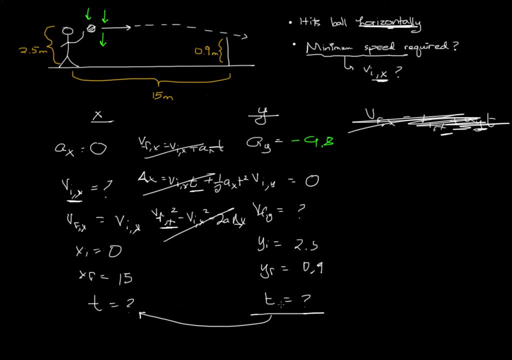 both sides. It's really not an x variable or a y variable, It's both, and that's why we kind of just put it on both sides. So whenever you're kind of stuck like this, see if you can solve for time on the y side and then plug it into the 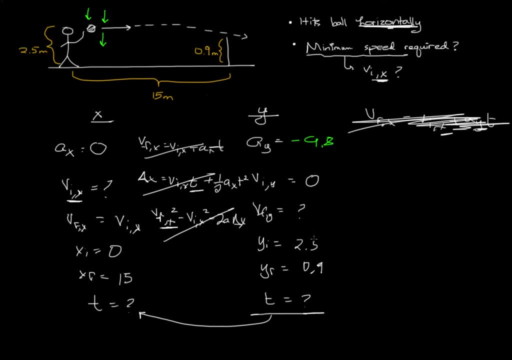 x side, or vice versa, depending on your situation. So let's see, can we do that, Can we solve for time on the y side, And we can. So what should we use? We can use: delta y is equal to vi y. Let me write this more neatly: Vi y. 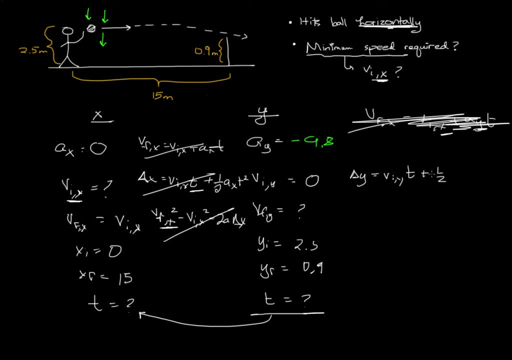 t plus one-half, a y, t squared. Okay, And let's see delta: y is final minus initial, so point this is 2.5, so 0.9 minus 2.5, which would get you negative 1.6.. Equals 0 plus one-half. 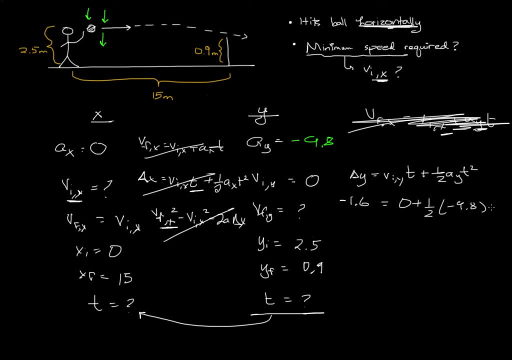 times negative, 9.8 times t squared, And if we solve for time, we will get 0.57 seconds. So we got time, Now we can plug, we can say: this is no longer question mark, Now we know, this is 0.57, and this is 0.57. here And now can we use one of these three equations?